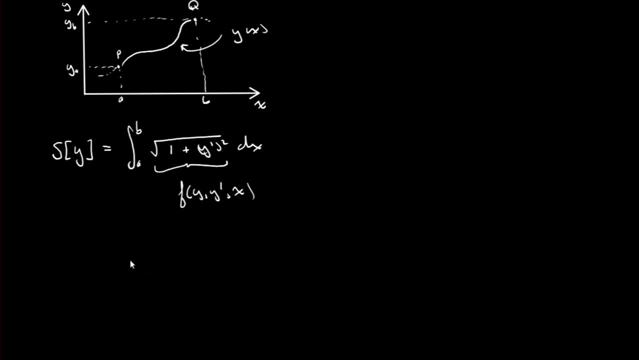 And this is what's going to appear in the Euler-Gronge equation. Well, without further ado, let's just go on and solve the problem. So we have: F is equal to root, 1 plus Y prime squared, And we aim to solve the Euler-Gronge equation for this problem, which is say 1 plus Y prime squared. 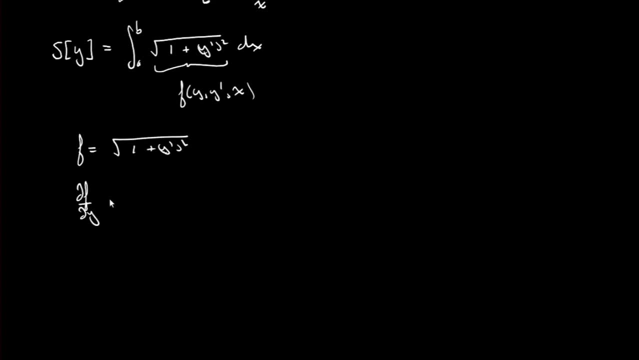 And we aim to solve the Euler-Gronge equation for this problem, which is say 1 plus Y prime squared. And we aim to solve the Euler-Gronge equation for this problem, which is say 1 plus Y prime squared. 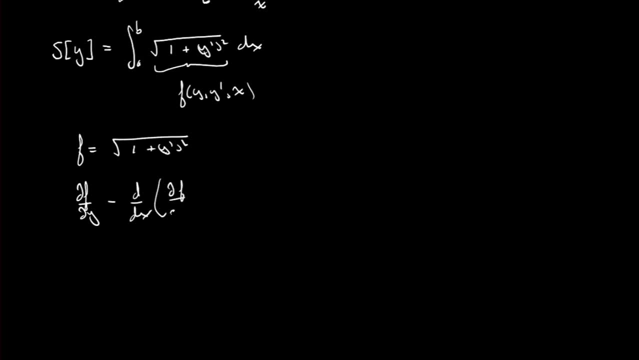 But instead of this component構 is a bit more involved, because really we're trying to differentiate with respect to y prime, 1 plus y prime squared to the half, and this has just got to be a half of 1 plus y prime squared to the minus a half. so we've multiplied by the power and reduced the power by 1. 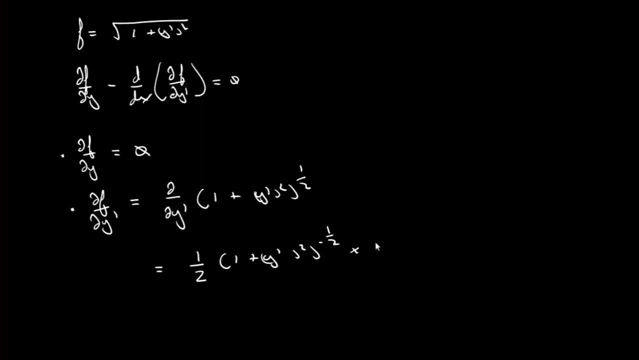 and then we multiply the whole thing by the derivative of the inside with respect to y prime, using the chain rule, so that's times 2 y prime. we can cancel the factors of 2 and then, when we simplify, we're going to come out with just y prime divided by the square root of 1 plus y prime, squared okay, and really we just need to. 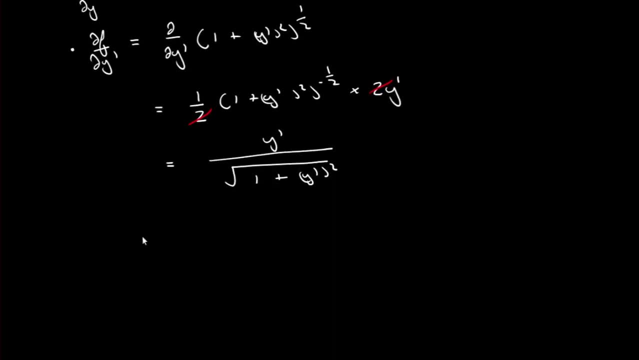 substitute these things into the Euler-Lagrange equation. so we put them in now and we're going to have 0 for df' dy minus. the total derivative of df dy prime which we just worked out was y prime over root 1 plus y prime squared. all that's got to be equal to 0 and of course you can probably see this is: 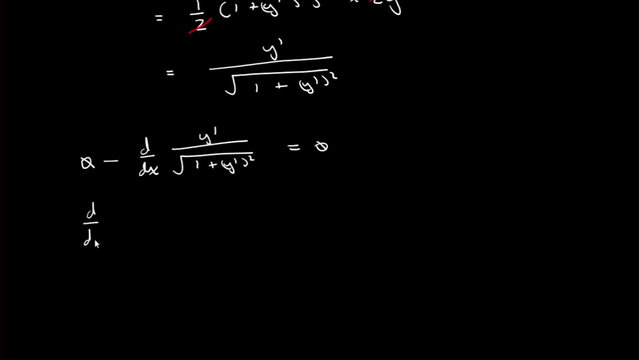 the same as the statement that the derivative, with respect to x, of y prime over root 1 plus y prime squared, which has got to be equal to 0. now, clearly, this is just a statement that y prime over root 1 plus y prime squared. what's? 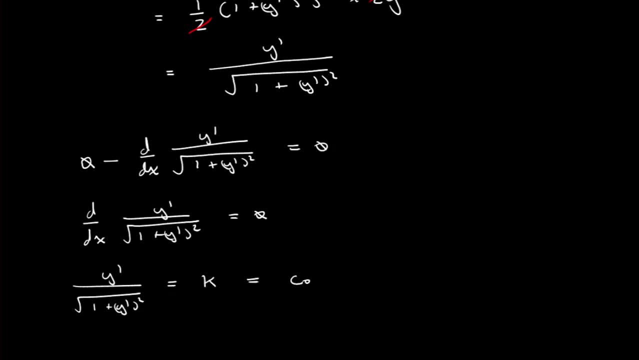 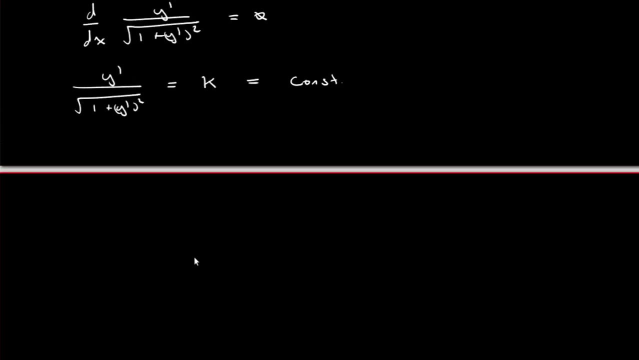 that got to be equal to equal to some constant case. okay, which is a constant right? and that's just clearly the same as the statement that its derivative is 0. the derivative of what is 0? a constant? what constant? any constant right. so now to continue. well, let's solve this equation. 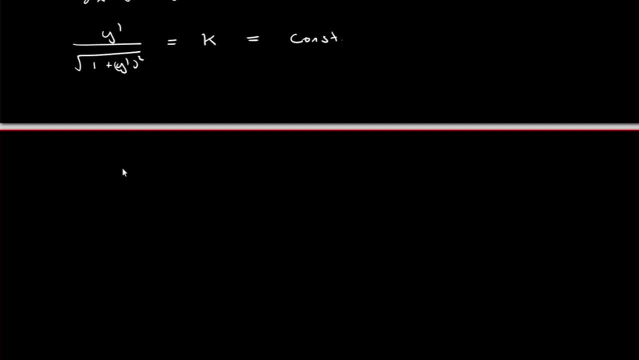 because the goal is here. there's a y prime here and y prime here, so really we'd quite like to collect them together before we begin solving the differential equation. so we multiply through by that root 1 plus y prime squared on the bottom, and we'll come up with: y prime is just equal to k lots. 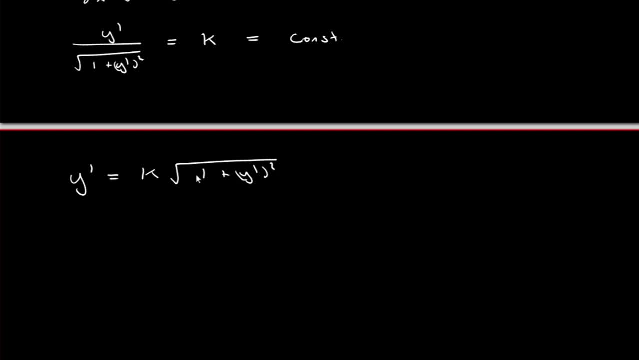 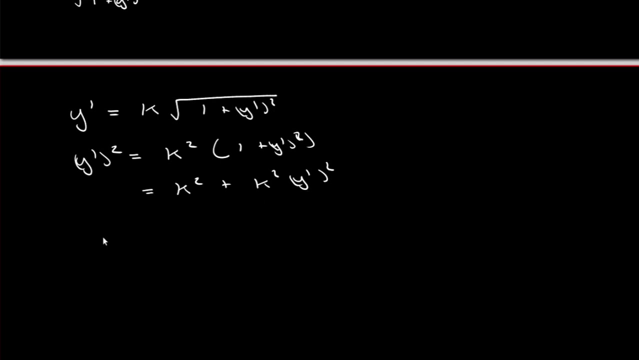 squared. we square both sides and to get rid of the square root and we'll come up with y prime squared. it's just k squared 1 plus y prime squared, which is just k squared plus k squared, y prime squared. now, if we just move all of the y prime squared to the left hand side, we're going to come up with y prime squared times. the 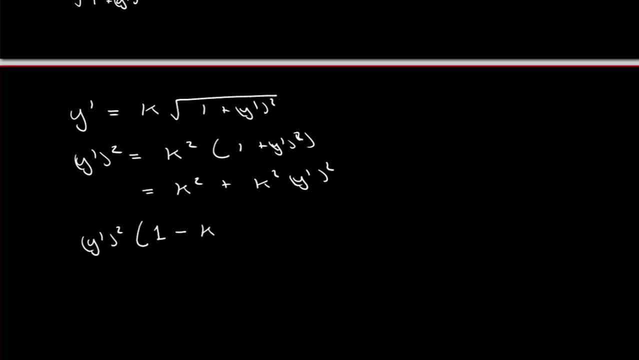 contribution of 1 from this side, minus the k squared from that side. so this came from here and this came from, came from, came from here, then it's going to have that's going to be equal to k squared, which is what's left over. and, of course, well, we're on the within our rights, just write y prime, it's just. 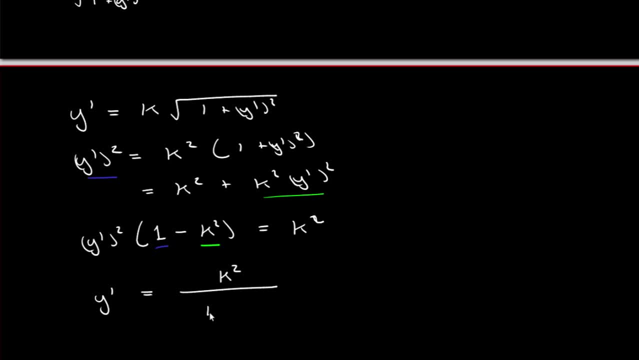 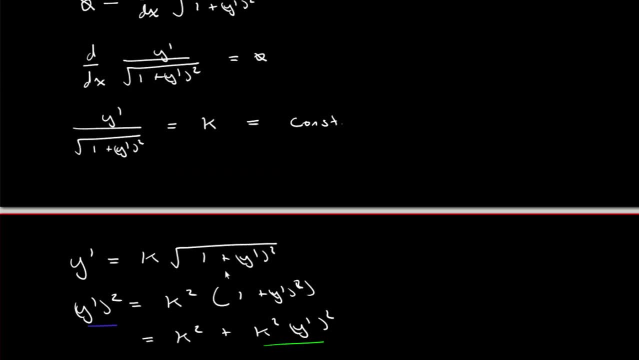 equal to the square root of k squared over 1 minus k squared. so that's going to be equal to k squared. so the square root of that particular is plus or minus that, but this thing, k. we said that was a constant, remember. so the square root of k squared over root over 1 minus k squared, that's just. 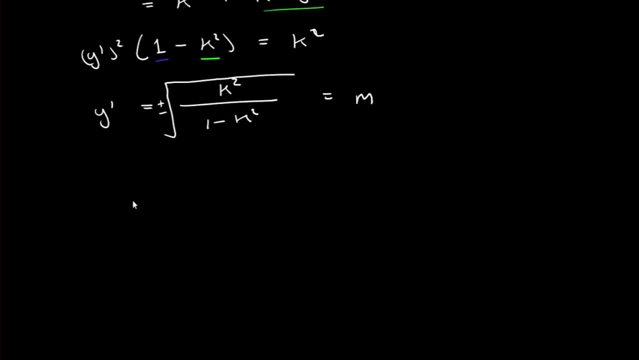 another constant that we'll call m. okay, so well, we have y. prime is equal to m, so the derivative is equal to m, and if we integrate that, what we're going to find is y is just equal to mx, plus some constant, and this is just the equation of a straight line. so we've proven what we set out.